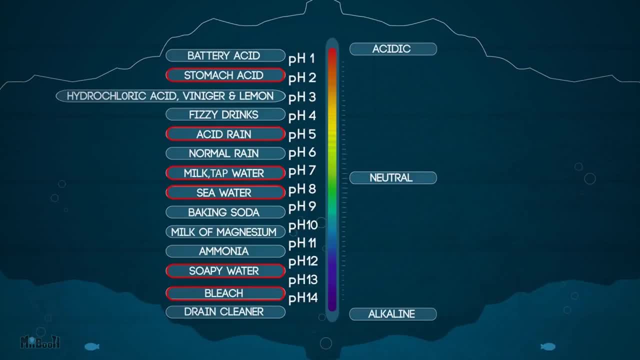 The lower the number on the pH scale the more acidic the solution is. And the higher the value the more alkaline the solution is. And 7 is the neutral zone. 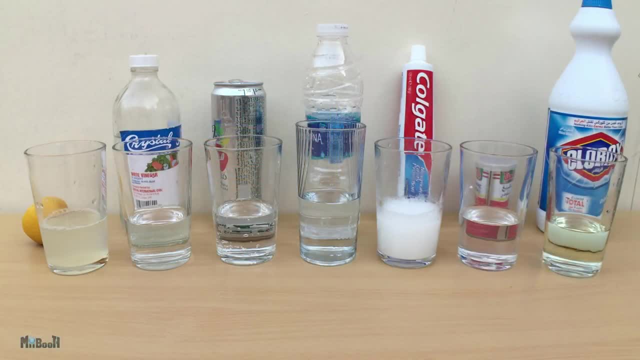 Here are 7 commonly available solutions which we are going to test. Lemon juice, vinegar, carbonated lemon soda, water, toothpaste and water solution, baking soda and water solution. And finally bleach. 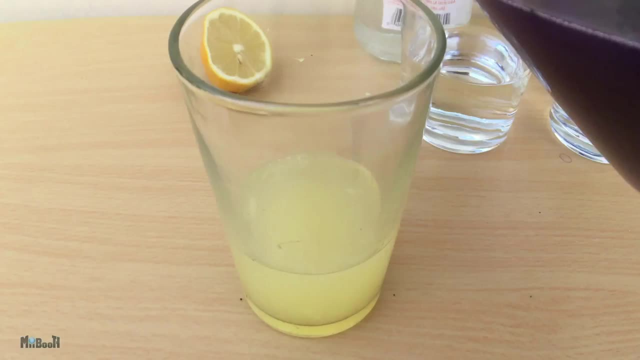 Now I am going to pour my indicator into the glasses to see what happens. The lemon juice being the most acidic of the lot changes to a bright red color. 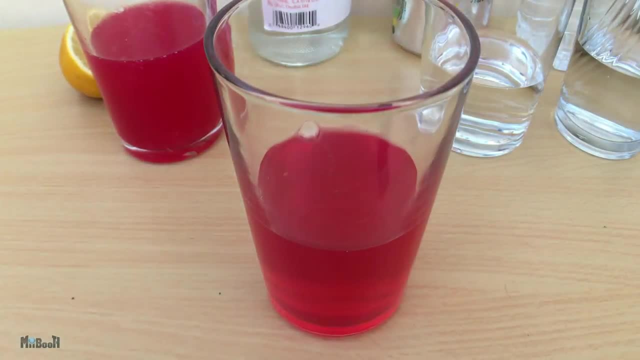 The vinegar changes to a pink or a less bright red color. The lemon soda changes to pink shade. 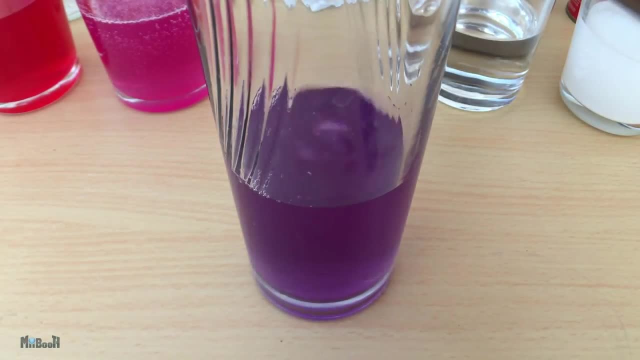 The water being neutral takes the color of the indicator and becomes purple. 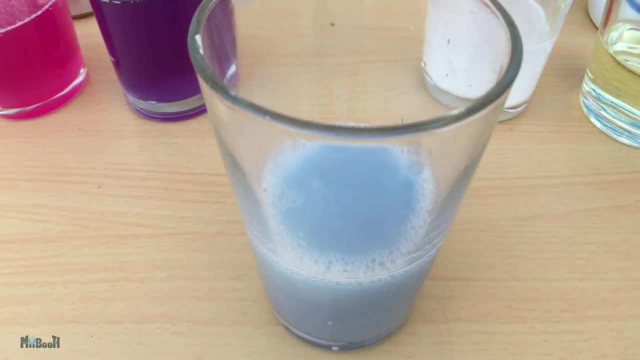 The toothpaste and water solution changes to a blue shade which means now we have stepped over to the alkaline zone. 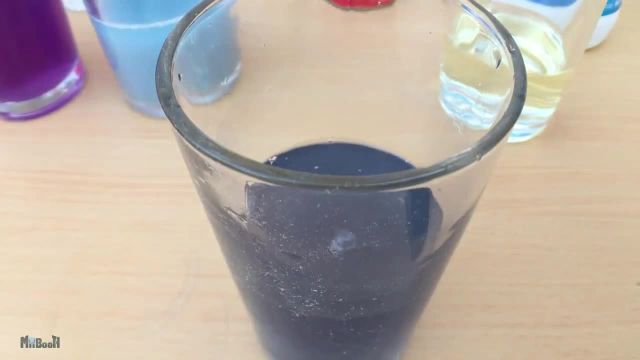 The baking soda and water solution turns a bluish green shade. 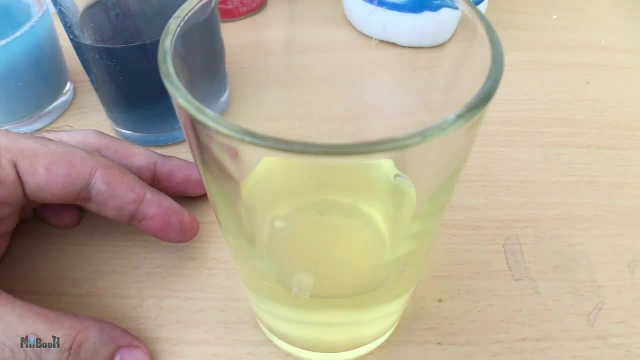 And finally the bleach being the strongest base of the lot dissolves the purple color completely and retains its own light yellow color. 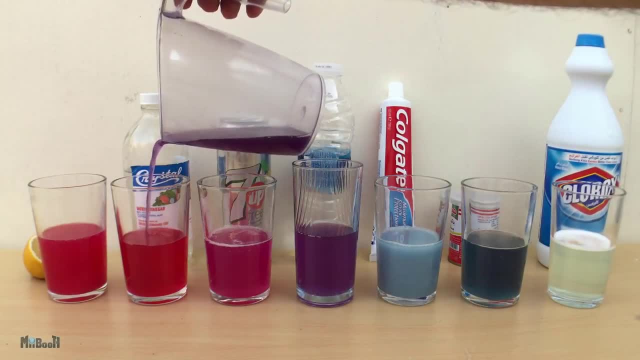 You can see how the indicator has changed color in all the different solutions. 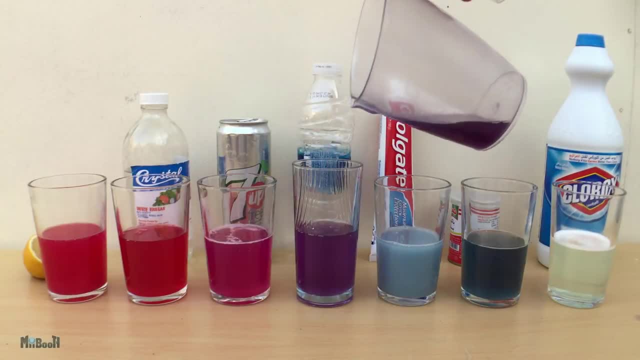 This is a very fun and easy experiment you can try at home for almost free and it is also an excellent and safe way to demonstrate the concept of acids and bases to kids. 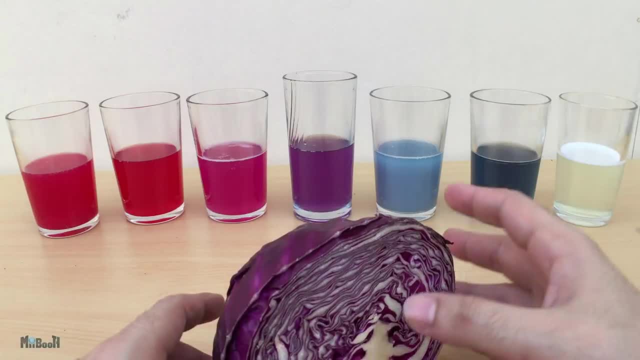 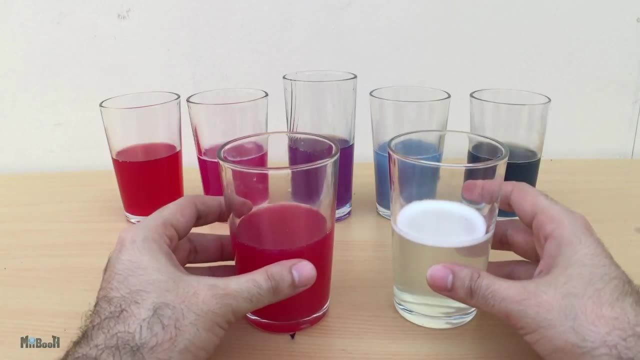 Now I was also told at school that acids neutralizes alkalis and vice versa. So that means if I mix the solutions at the extreme ends together they should cancel out each other and I should end up with a purple color. So let's try it. 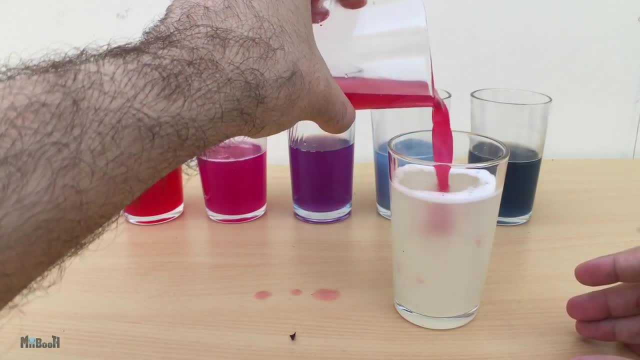 When I mix the lemon juice with the bleach there is no effect on the color. The bleach is a much stronger base than the lemon juice is an acid. 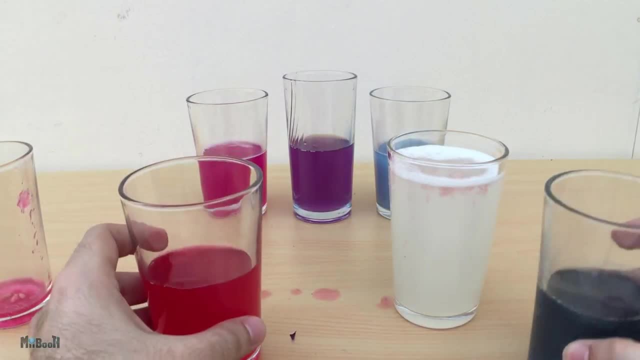 It will require a lot more of juice to neutralize the alkali completely and turn the color back to purple. 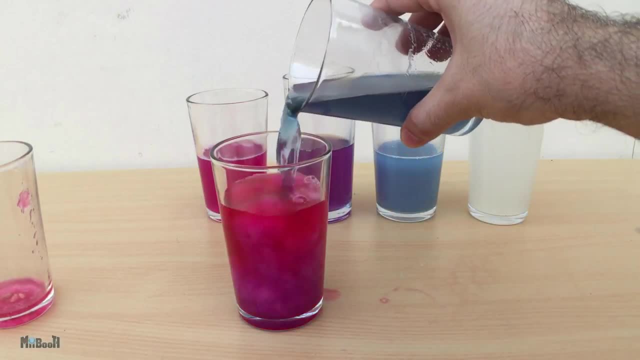 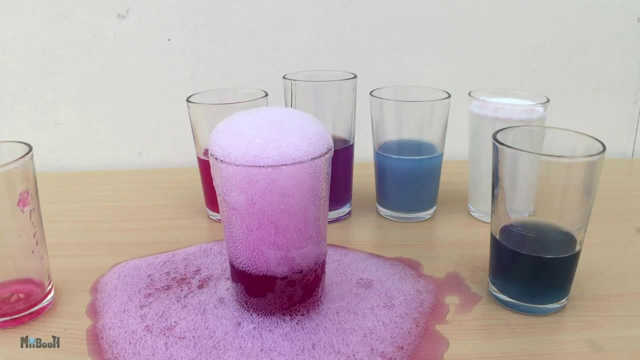 Next when I mix the vinegar and baking soda there is a sudden release of carbon dioxide gas and the whole solution foams and spills over the glass. It is still not completely neutralized so it is holding on to the pink color showing that it is still slightly acidic. 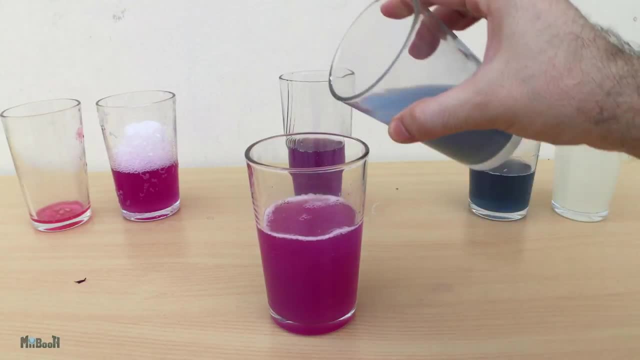 Finally when I mix the lemon soda and toothpaste solution both being a weak acid and a weak base neutralize each other completely and we get a perfect purple color. Same as the water solution.